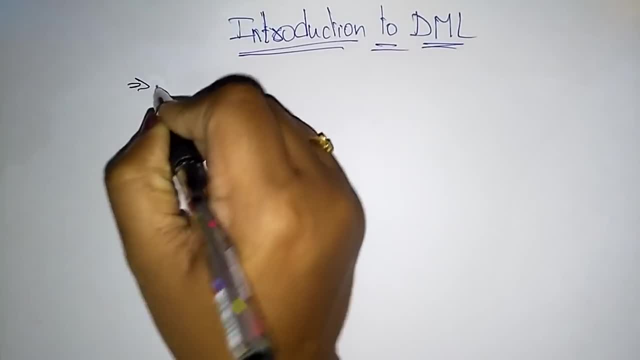 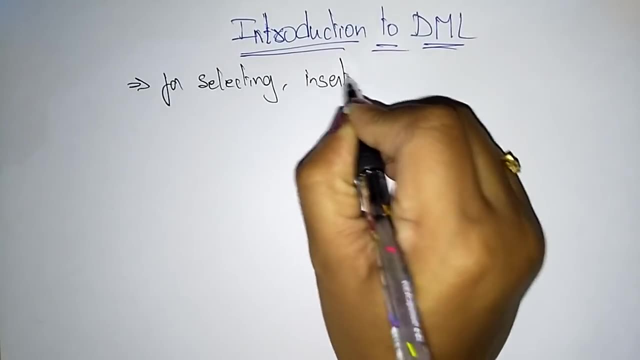 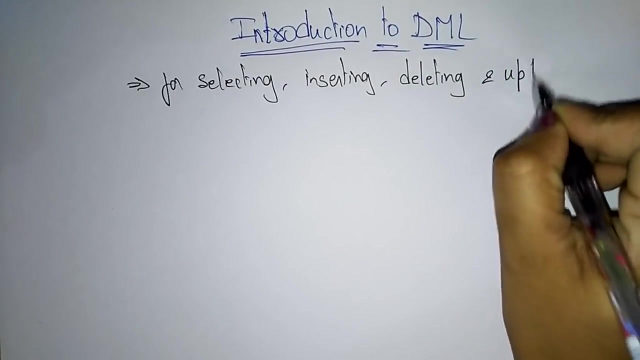 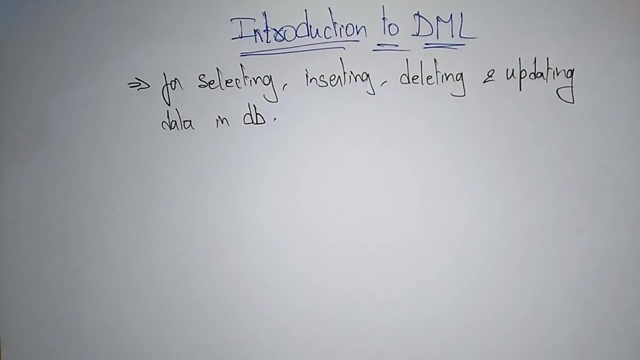 So the main use of data manipulation language for selecting, inserting, deleting and updating data in database. So to manipulate the database we need to select or to insert, delete or update. So it is used to retrieve and manipulate data in database. 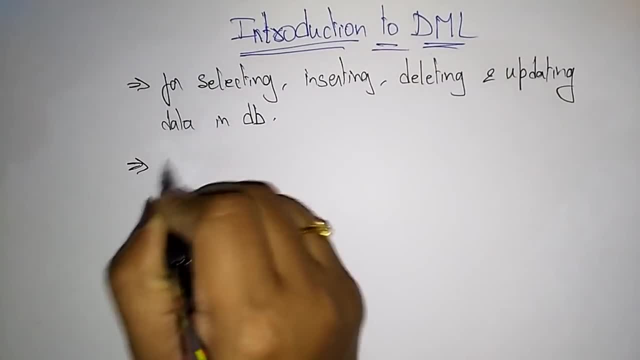 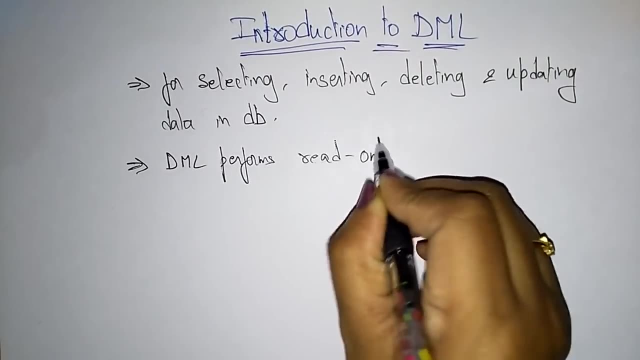 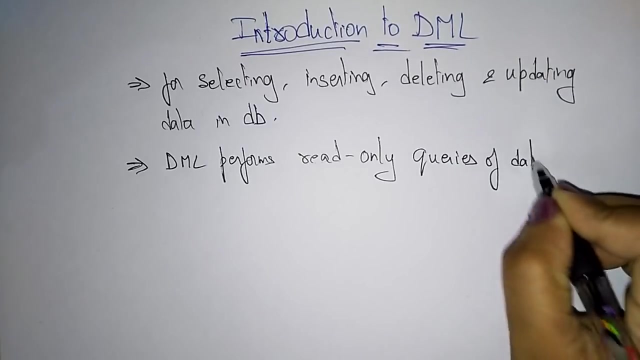 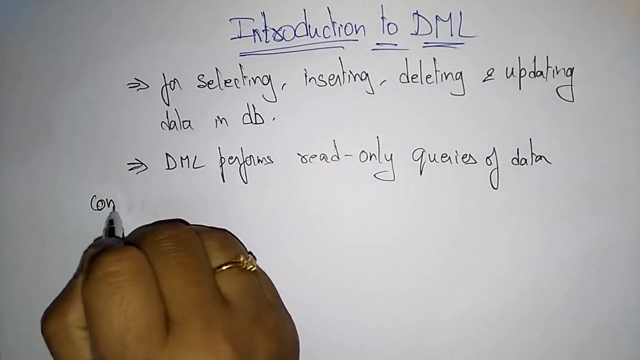 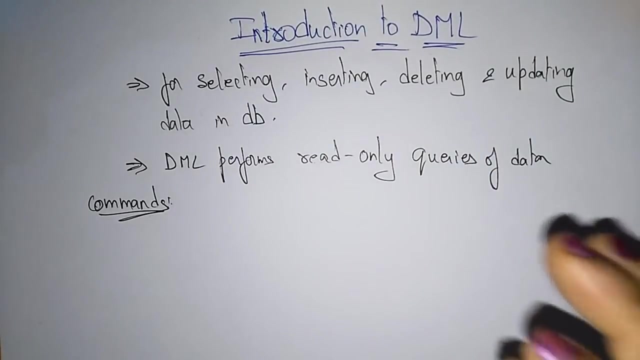 And one more thing here is data manipulation language performs only really read-only queries. It performs on only read-only queries of data. Okay, So this is about data manipulation language. Let us see what are the different commands that are used in the data manipulation language. The one thing you have to be remember: for manipulation language, we use select, insert, delete and update. So whenever you ask which type of language is used, we use select, insert, delete and update. 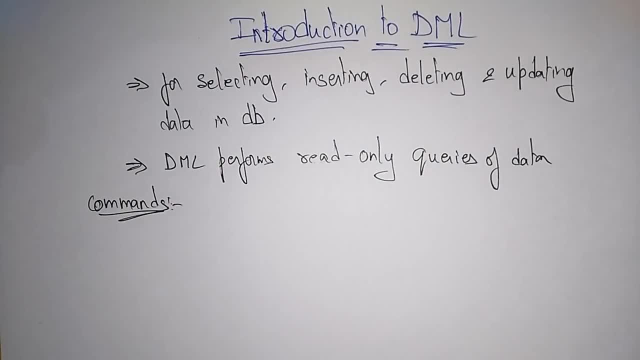 Now Цеet-начeste, data manipulation language is created, means you have to tell it that it is a data definition language. it is the rename or truncate. Those are all the data definition language commands, the commands, Whereas data manipulation commands are select, insert, update, delete. so the four are the data manipulation languages. Then you need to conserveтерес, southeast, update, delete and execute these all. 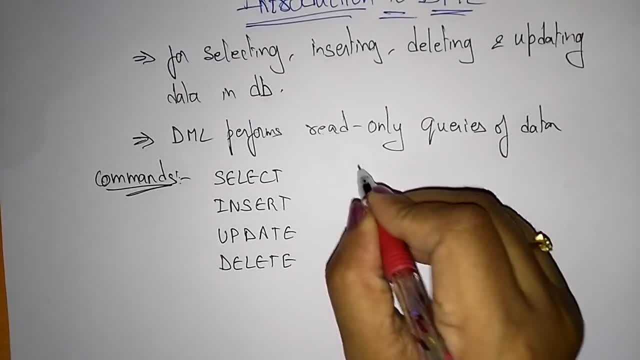 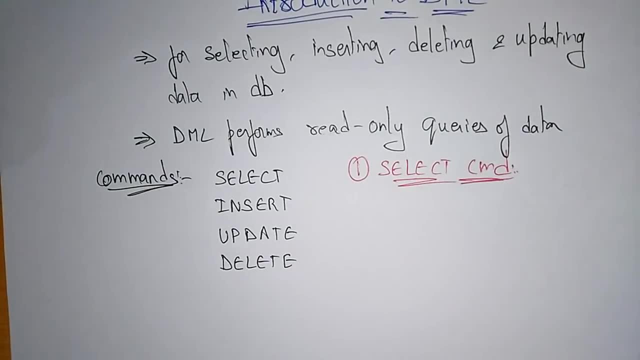 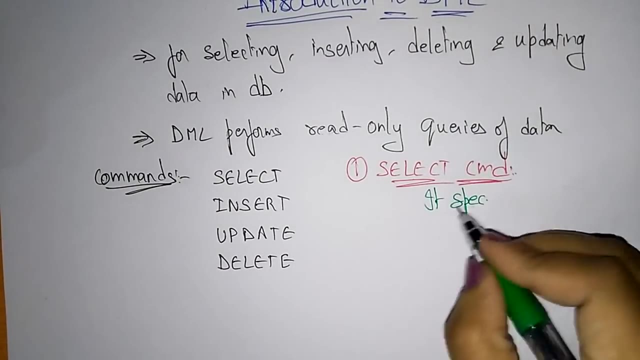 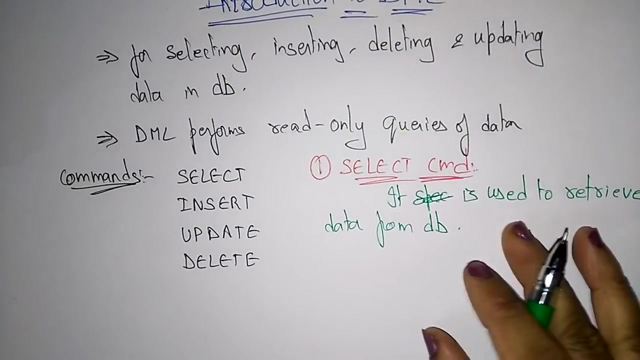 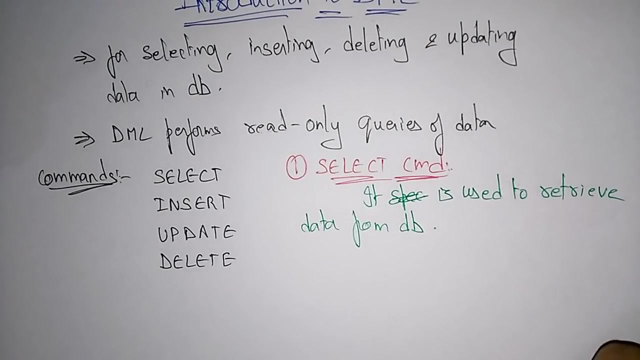 Let us see one by one. So what is the first one? So first one is the select command. So mainly the main use of the select command is it specifies: so it is used to retrieve data from database. So the main use of the select command is it is used to retrieve data from database. So in the select command we use different clauses. So the clauses that are used in the select command are: so the clauses are where clause. 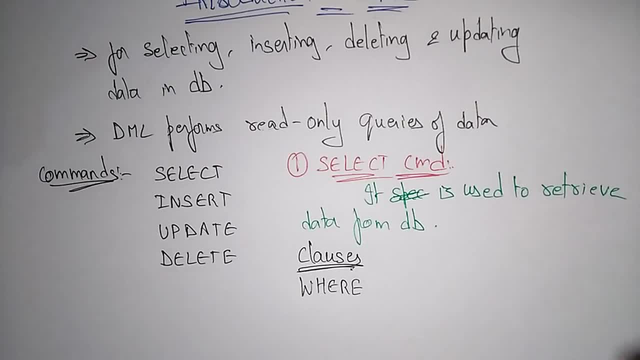 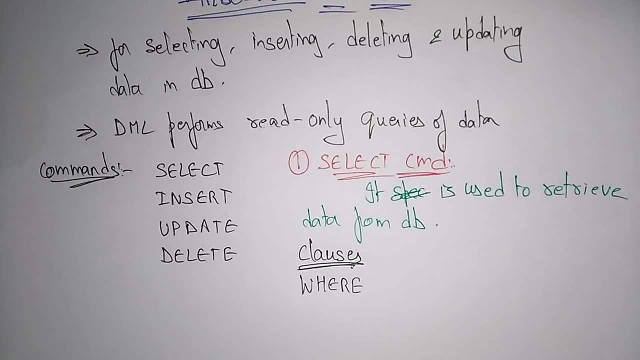 So if you want to select any query, if you want to select a particular record, you have to mention the condition from where you have to select Means, from where which condition has to be satisfied. So the select command will use different clauses. Those clauses are where group by having clause, order by order by and as clause. 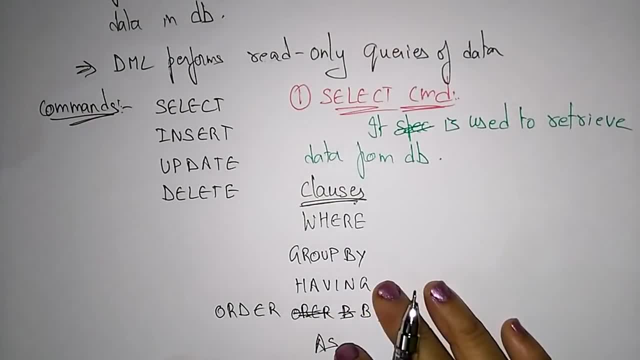 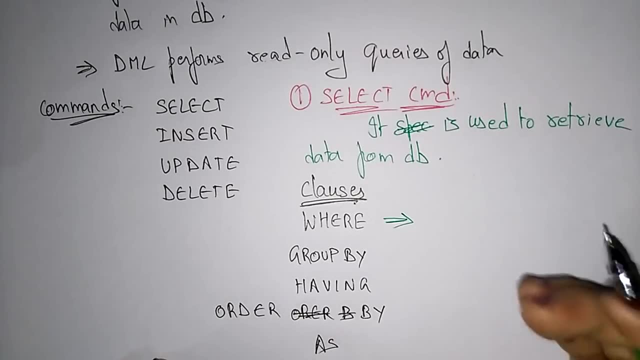 So these are the different clauses that are used in the this this select command. So what is the where clause will do? So where clause specifies which row to retrieve- Okay, Specifies which row to retrieve What this group clause will tell. 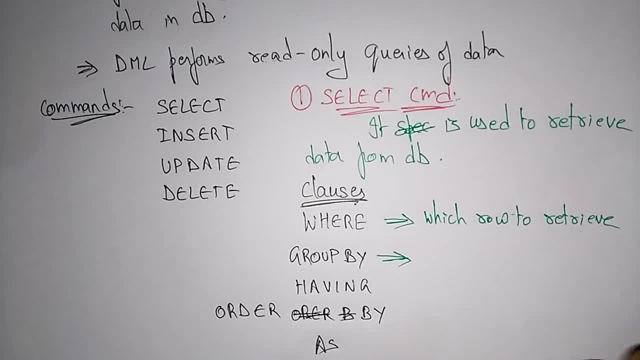 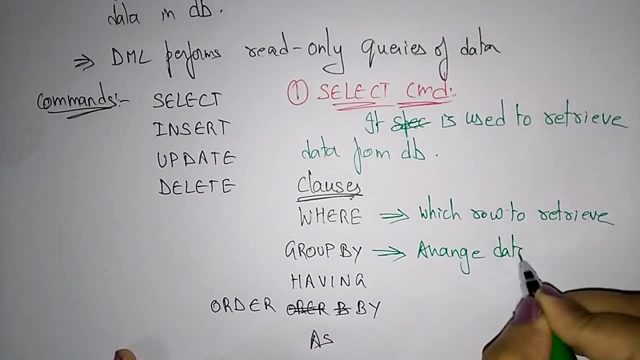 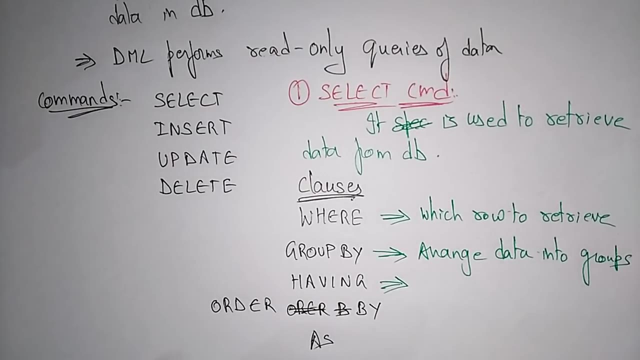 The group clause will select. it is used to arrange the data into groups. Use it to arrange data into groups. And what about the having clause? Having clause is used to select among the groups defined by the group by clause. It selects among: 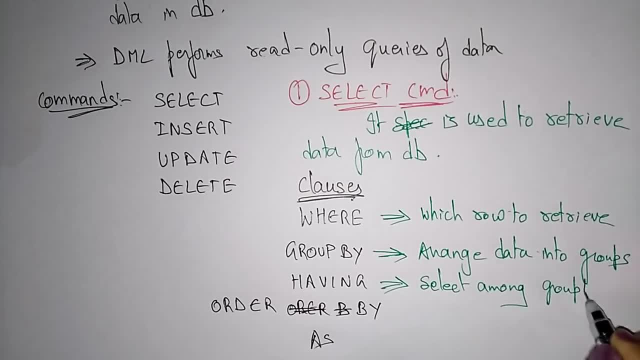 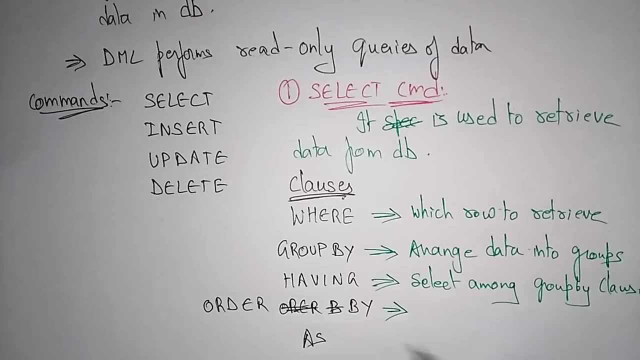 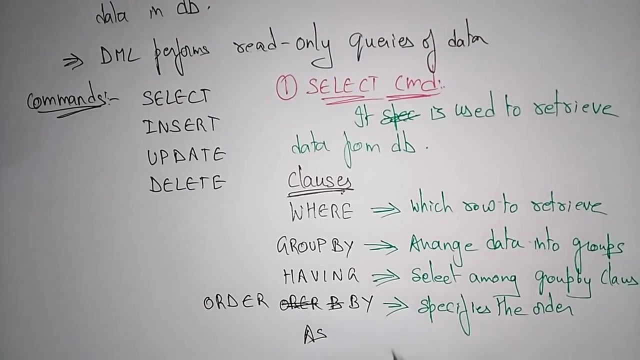 defined by group by clause, Among group by clause. Then what about the ordered by clause? So the ordered by clause specifies an order in which to return the rows, Specifies the order In which order the rows has to be appeared as an output. 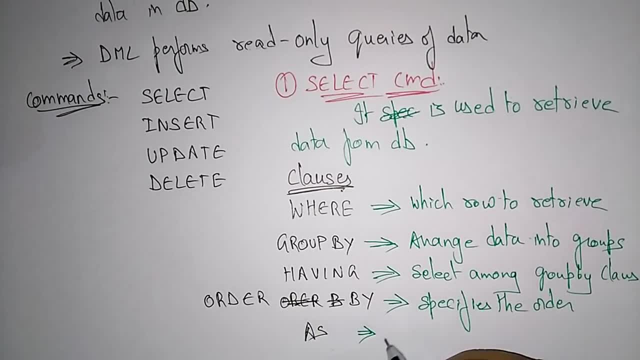 So that will be tell by the ordered by clause. Whereas as clause it provides an alias which can be used to temporarily rename tables or columns, It gives just alias Or rename tables. So these are the different clauses that are used while you are writing the select command. 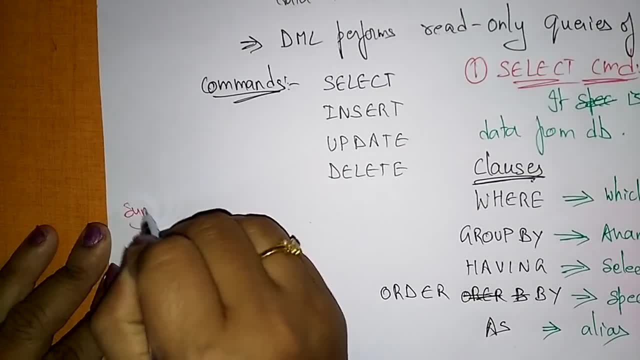 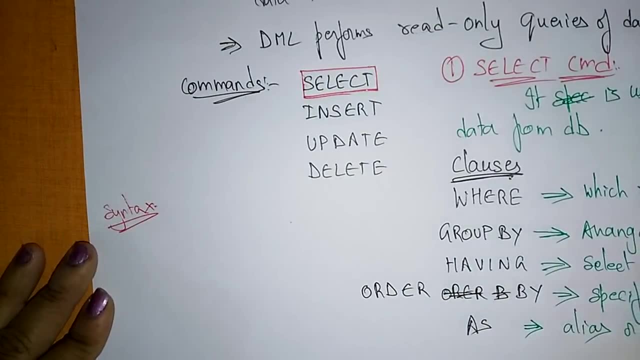 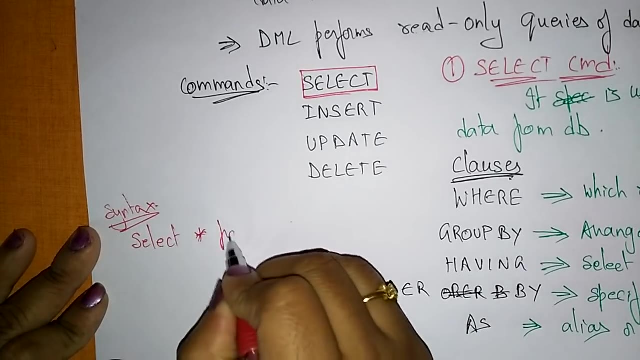 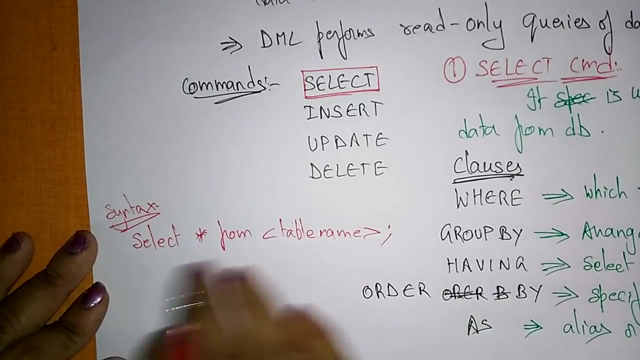 So let us see what is the syntax for the select command. So we are just discussing about the select in data manipulation language. So let us see the syntax Select star from table name. So this is the syntax. Suppose if you have written select. 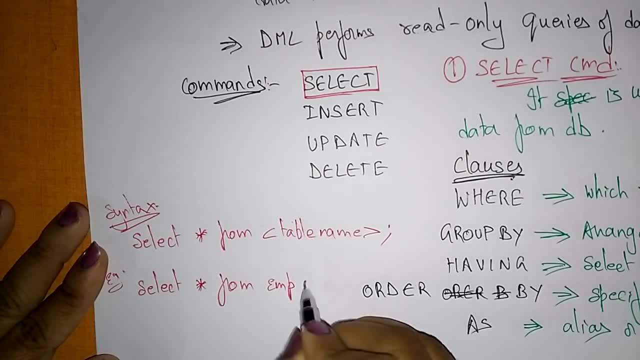 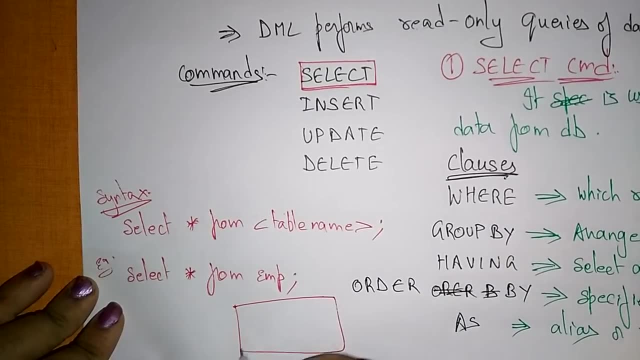 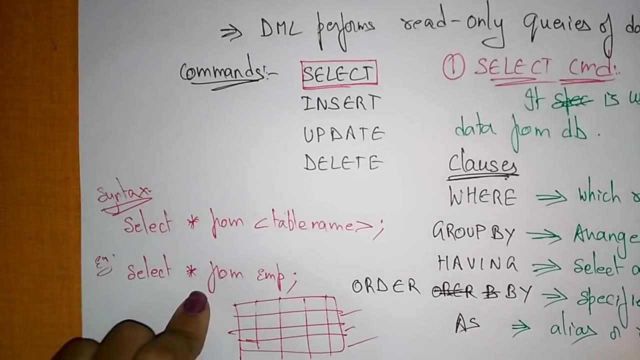 star from employee. So in the employee table it returns all the rows. So complete table will be appeared on the screen. Means it returns all the rows in the table. So the star indicates all the rows that are present in the table. That has to be selected. 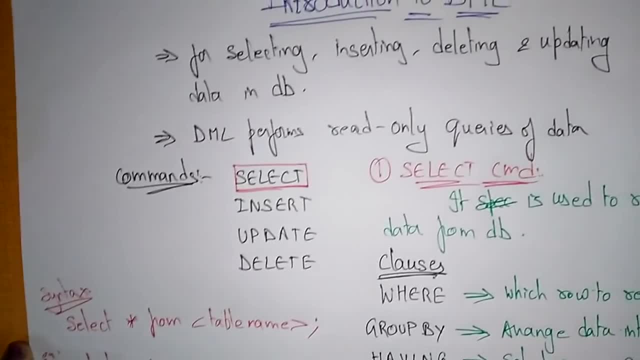 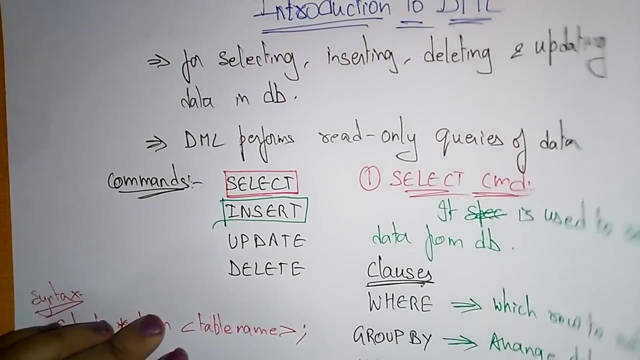 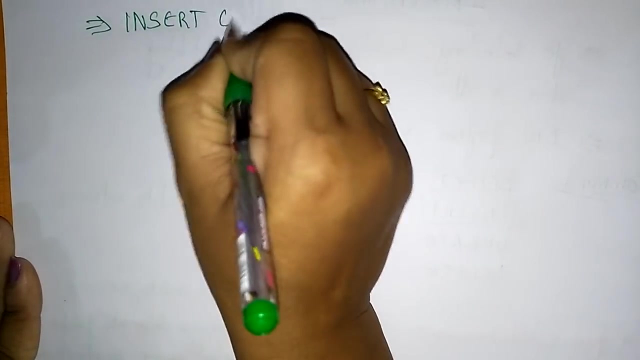 So that the year. This is the syntax for the select command. Now let us see the next command. What is the next command? So next is the insert. So let us see what is the insert command will do So. insert command. 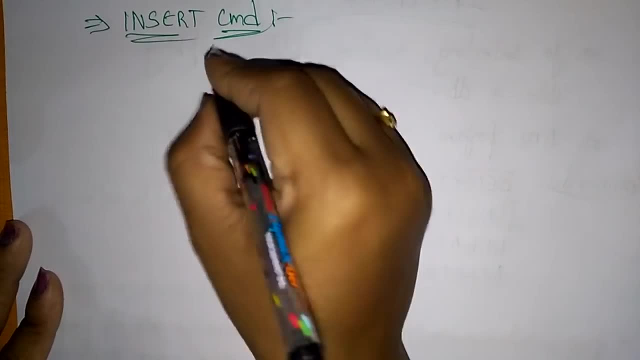 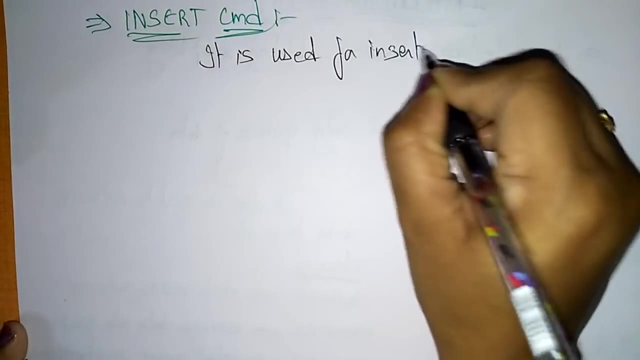 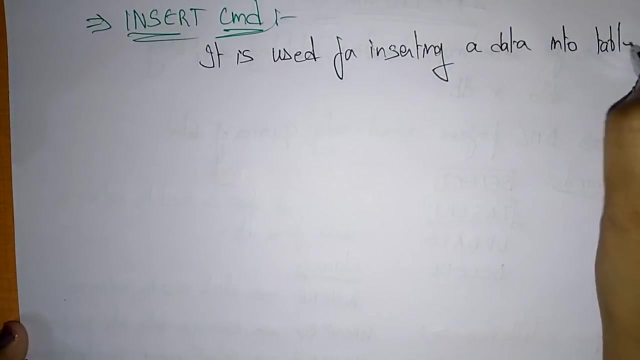 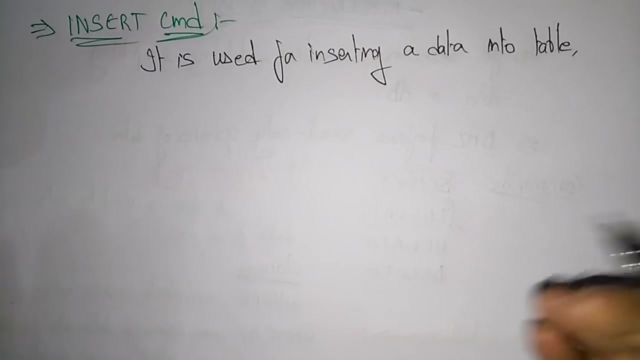 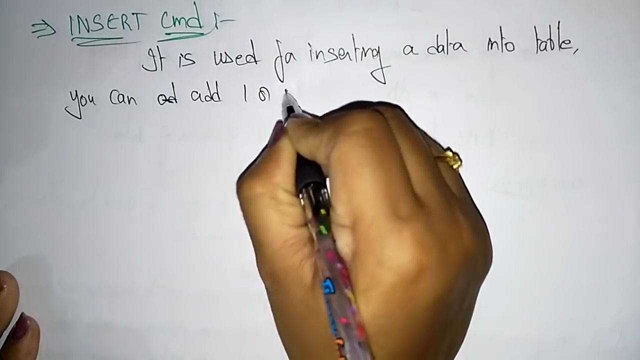 What you will do is insert command. command is used for inserting data. it is used for inserting a data into tables. you can add one or more records to any single table. if you want, you can add one or more records. you can add. add one or more records into a single table at a. 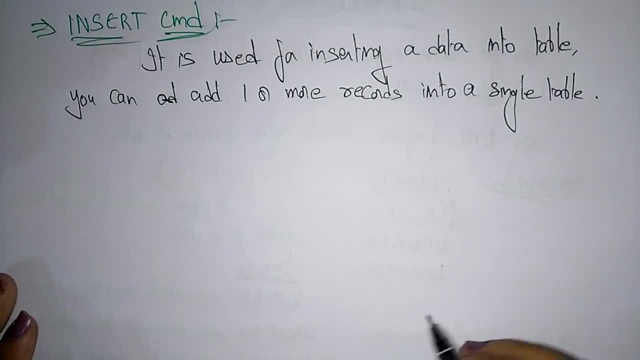 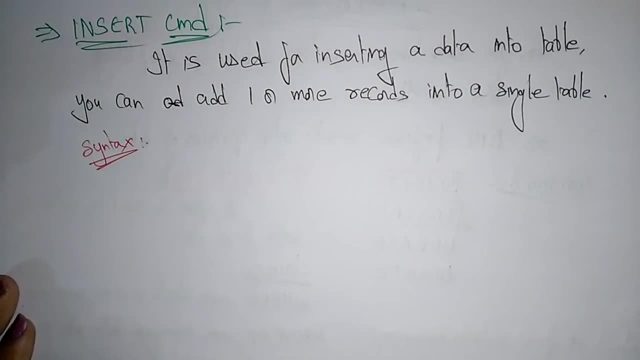 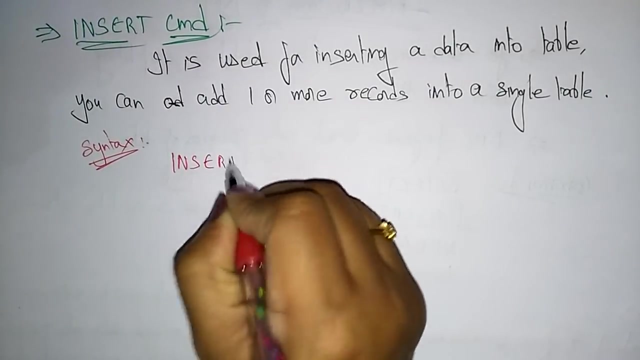 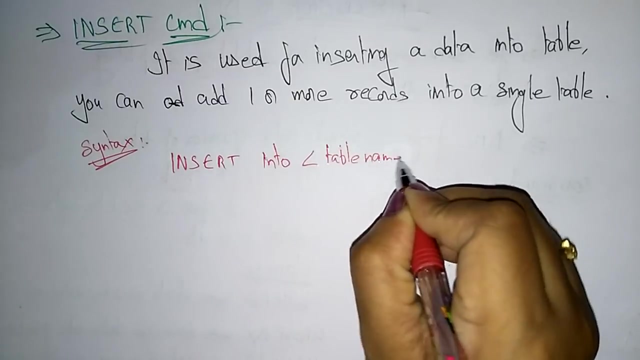 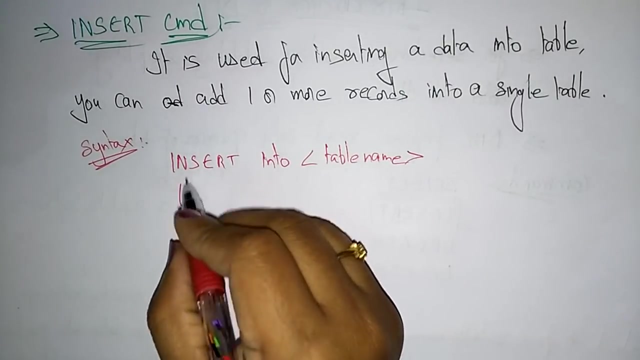 time. okay, in a single table. now let us see what is the syntax for the insert command. so insert is any comma, is a command that is using the data manipulation language. insert into where you have to insert. so you have to mention that table name, okay. so insert into table name. so here you have to mention the what values means. 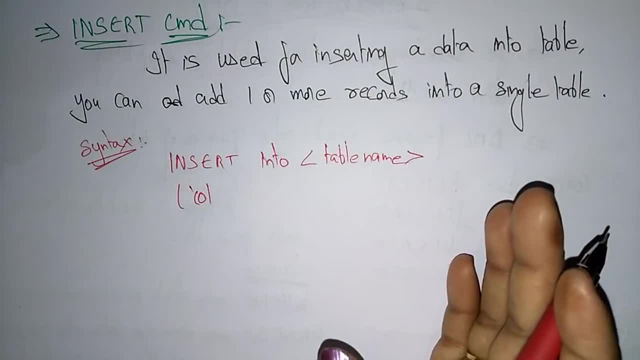 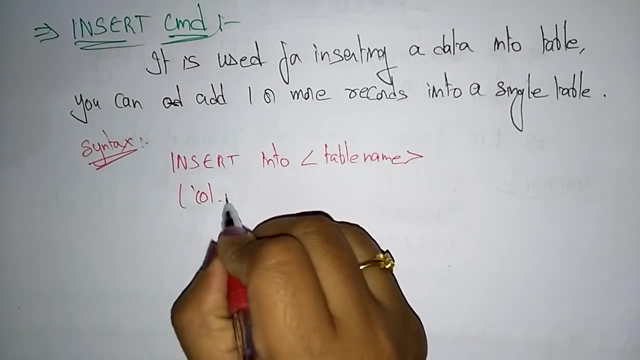 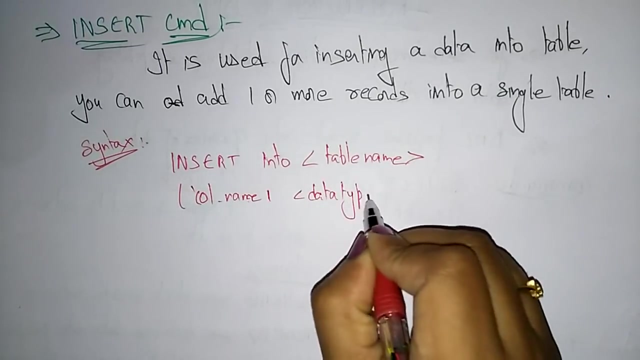 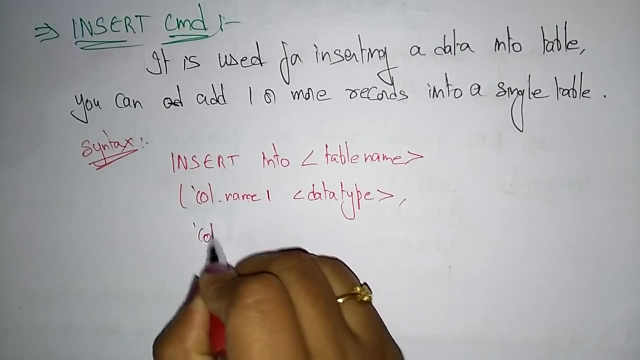 you have to insert in which field means, in which attribute or in which column. so you have to mention: insert into table name, column column name 1 and you have to mention the data type. suppose if you are taking an ID, ID ink like that and a column name to data type. 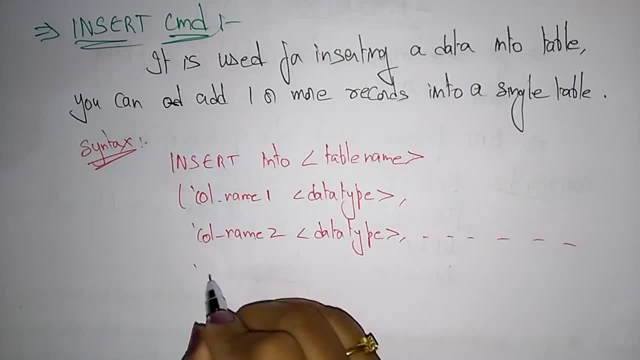 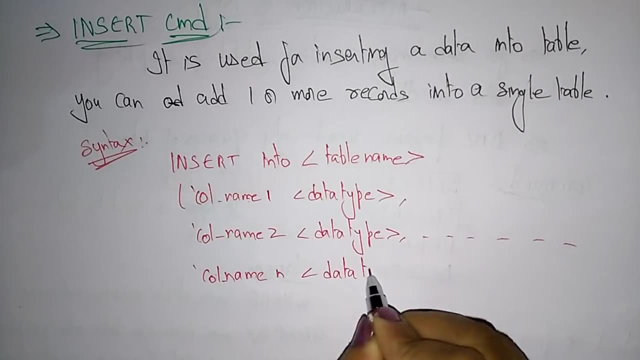 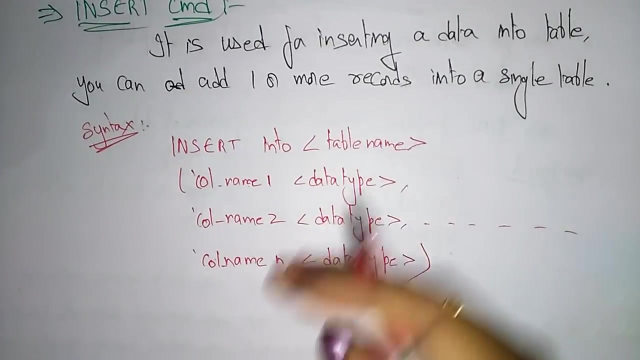 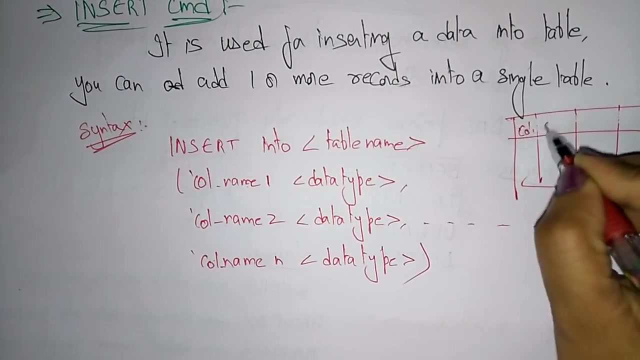 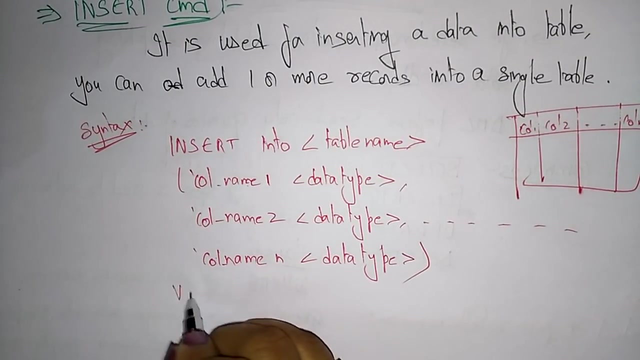 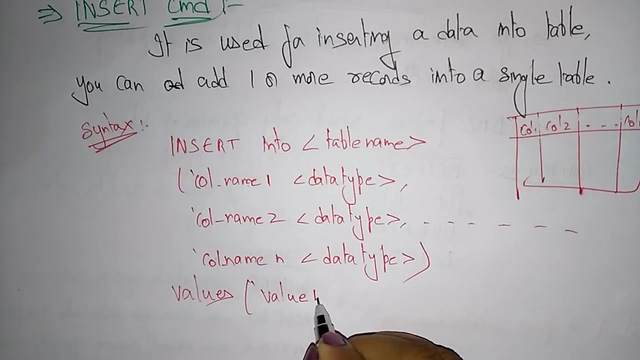 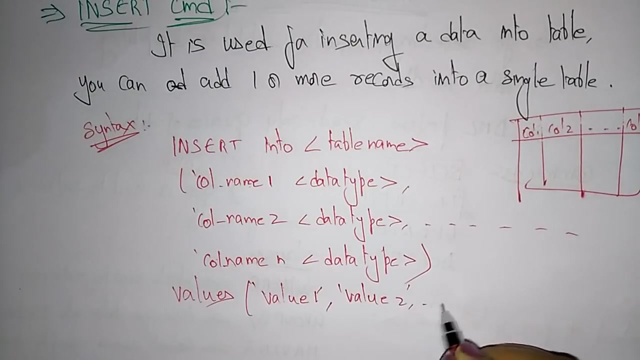 up to column name n data type. so close the columns, only up to here. that now, up to here. I created column names, column 1, column 2 up to column n, so now I want to insert values into that column values. okay, so you have to mention the value 1, value 2 up to: 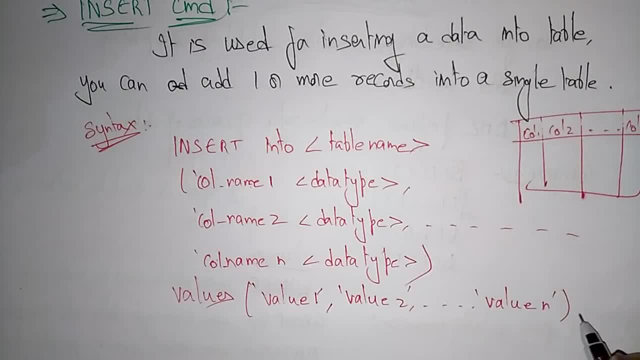 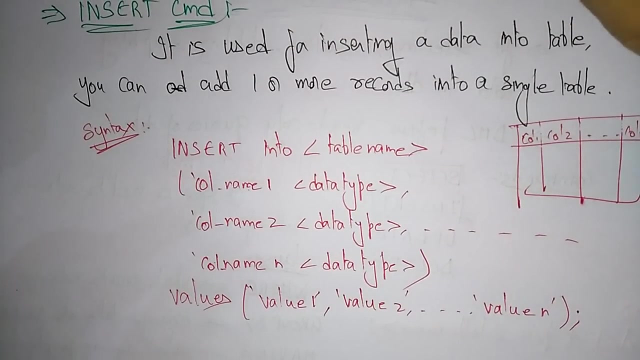 value n. okay, so this is about the insert command syntax. so you are inserting a values into that particular column record. so so, particular table. so let us see the next command. also, what is the next command? so before going to that next command, I'll just give a simple. 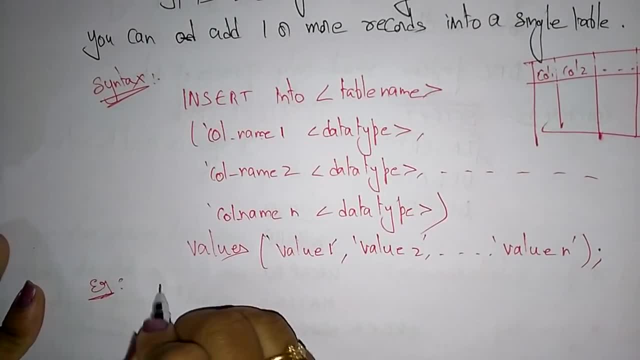 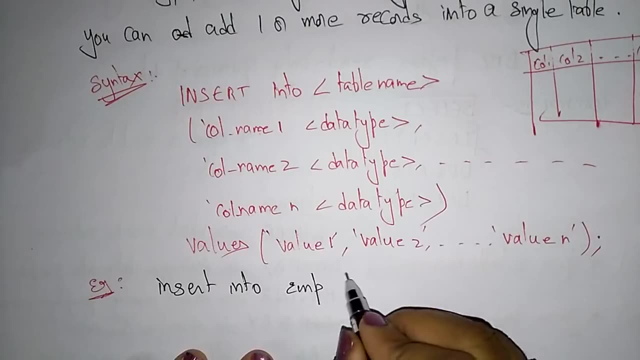 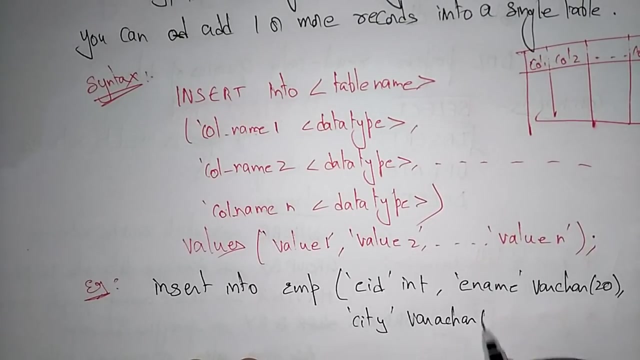 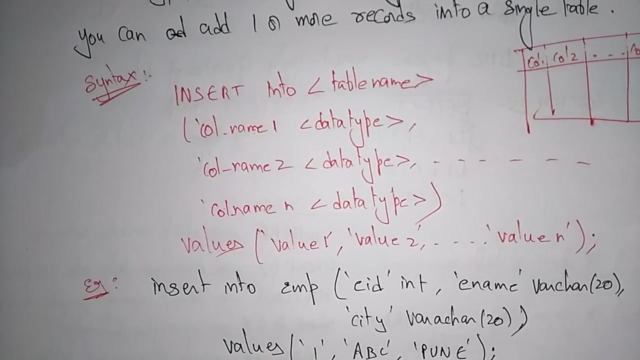 example for this. what is the example insert into? so the employee table, what I already created, so the study. so first is employee ID of data type int comma. employee name of data type worker and city data type: worker 20. so these are the. now I am inserting the values values: 1, ABC, Pune. so what it now the table look like this: 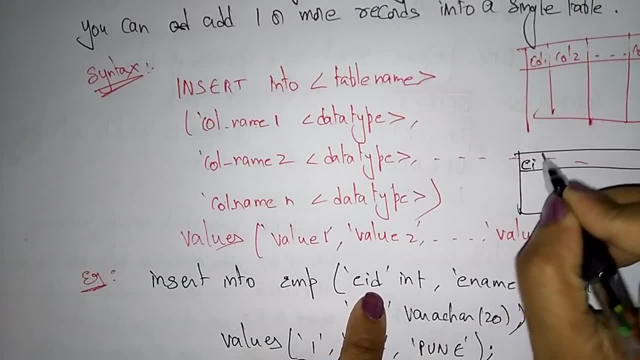 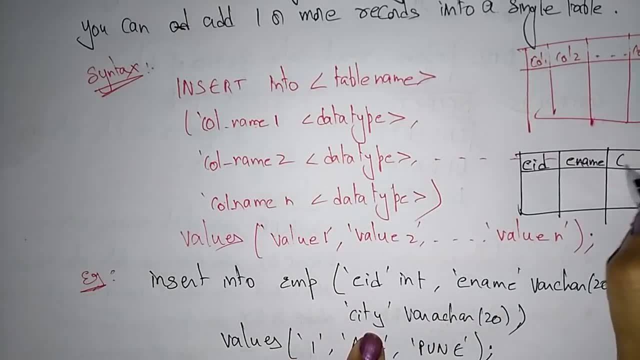 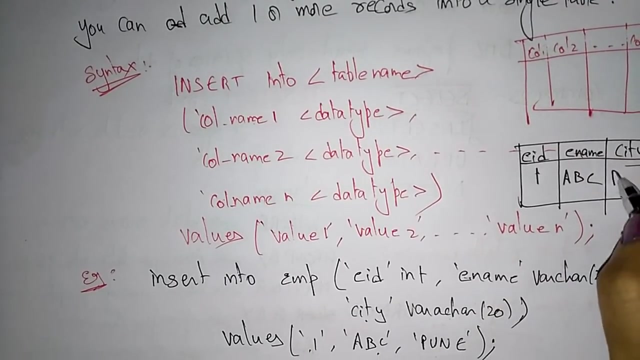 so first column is employee ID. so this is only the integer value you have to enter. next, employee name, next the city. so here the employee ID. the value I inserted here is a 1 and the employee name the value I inserted is. here is the ABC, and for city I insert the value as Pune. so this is how you have to insert as Pune values. 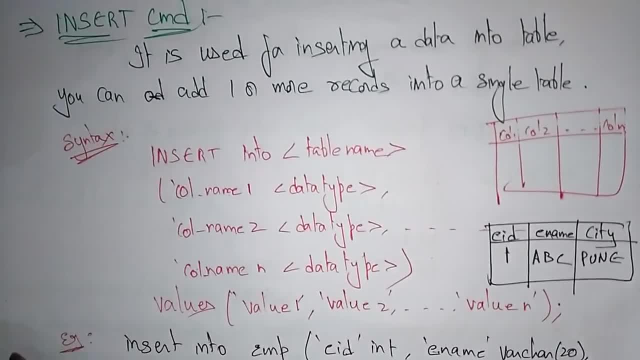 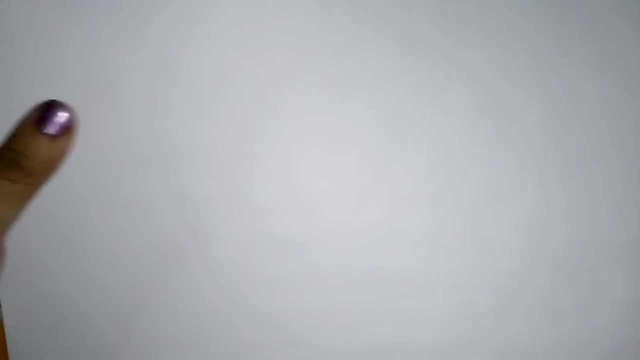 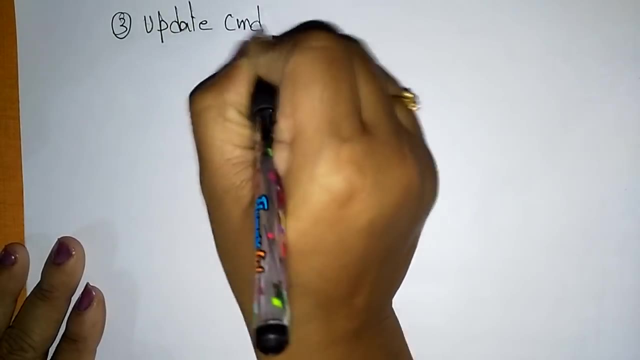 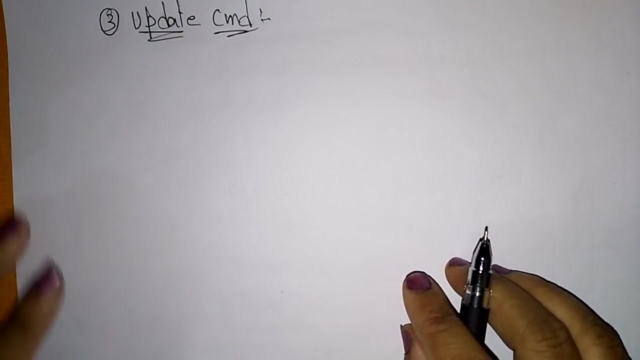 command is used. so now let us see the next command. so the next command is the update command. so the third command is update command. so we have seen the select command, insert command and, coming to the next data manipulation, language command, that is update. so what this update command will do. 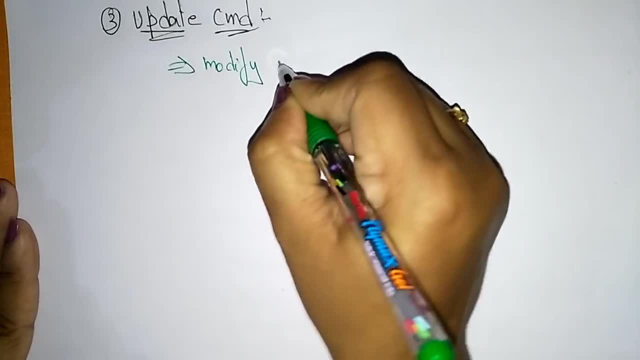 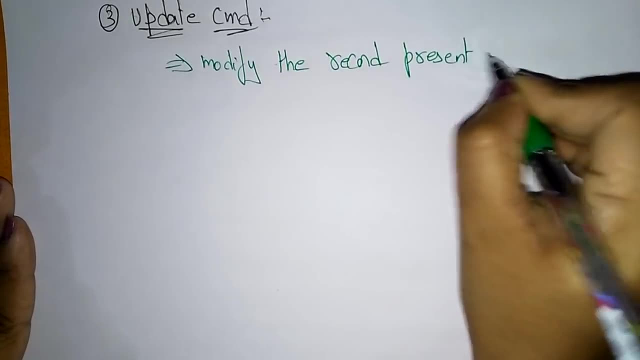 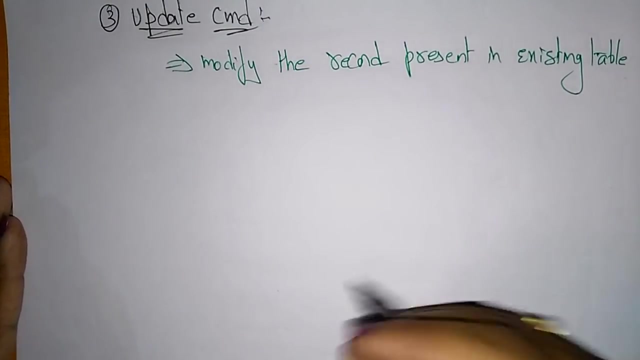 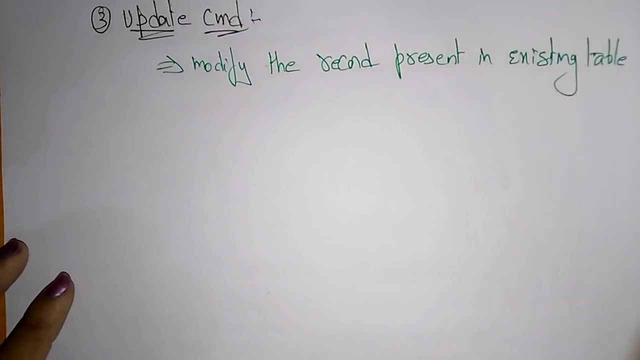 it modify. it modify the record present in existing table. so already the table was created, so on, and the values are also inserted. suppose if you want to update the record for the existing table, you have to use the update command. now let us see what is the syntax for this update command. 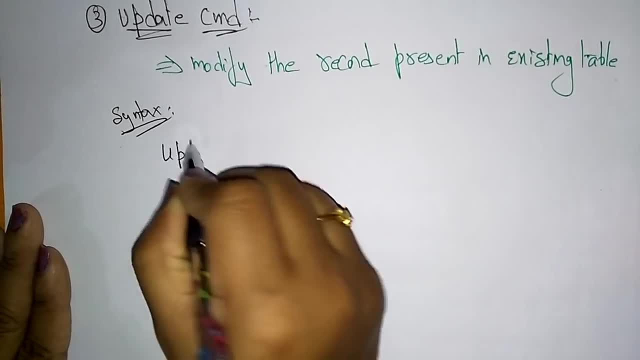 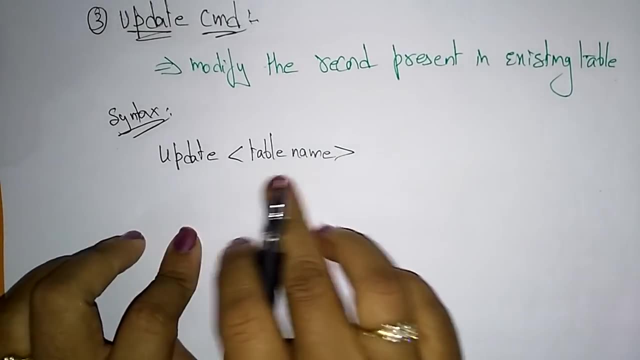 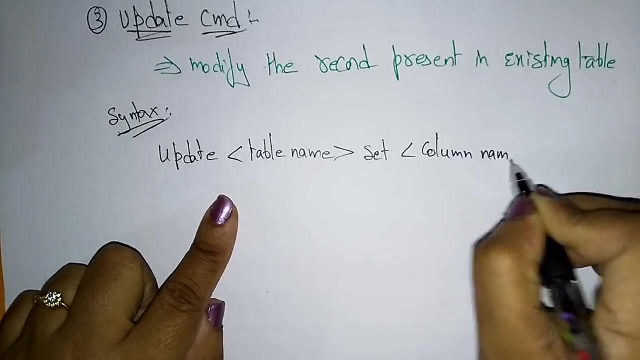 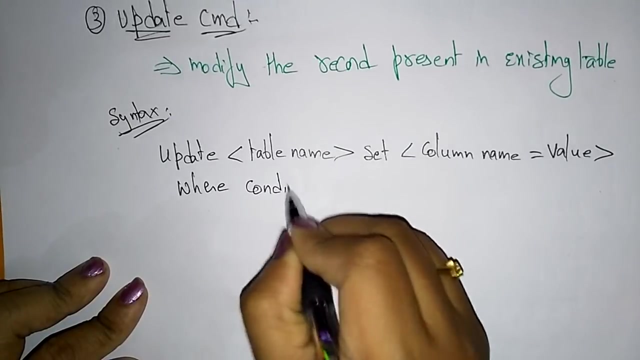 so update table name. so which table you have to be? update that table name. you have to mention here and now: set column name is equal to value, where condition. so this is the syntax for the update. now let us see the example for this, then you will understand. 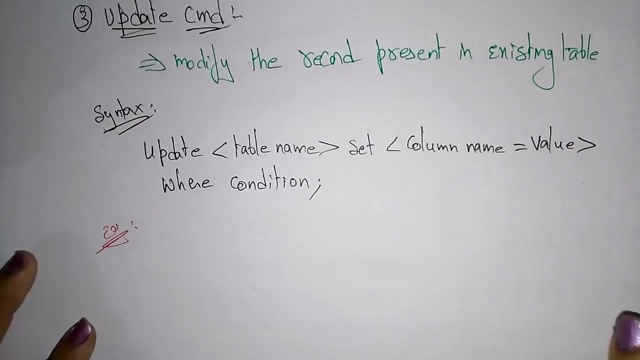 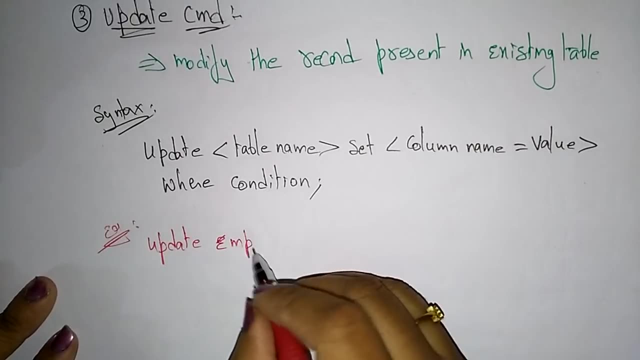 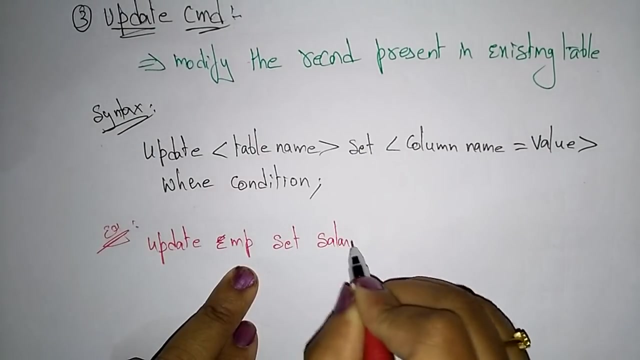 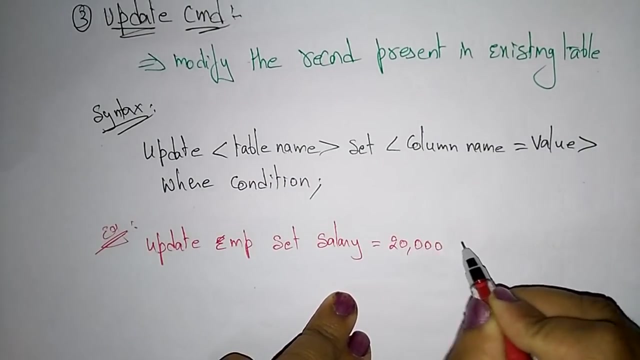 how this update command will update the table update. so now i want to update the employee table. so whatever i created, employee update, employee table set salary is equal to. so i want to set the salary 20 000 to the person where e name is equal to. 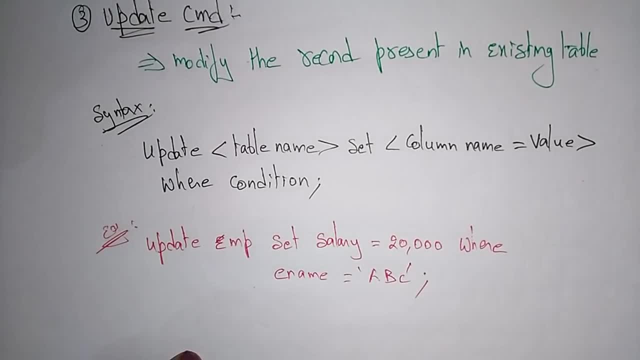 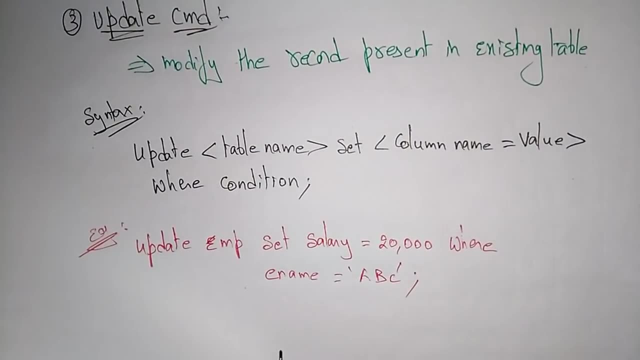 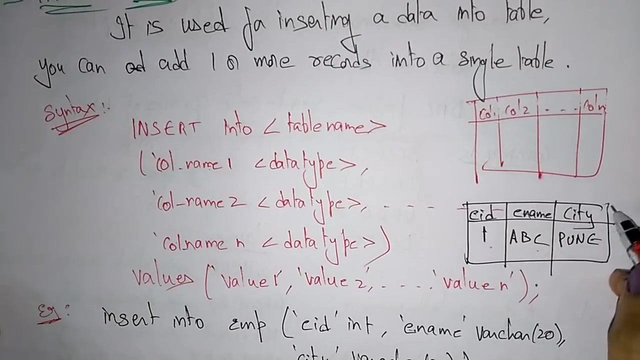 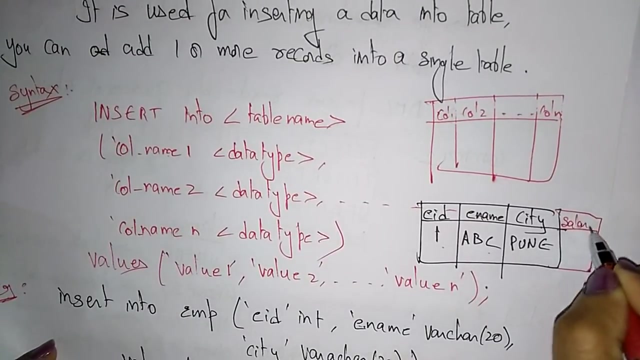 equal to abc. so i want to update the employee. i have to set this. i want to set the salary to that person where e name is abc. so previously i inserted these values. now here one more column will be added, that is salary. so here suppose i inserted salary also. 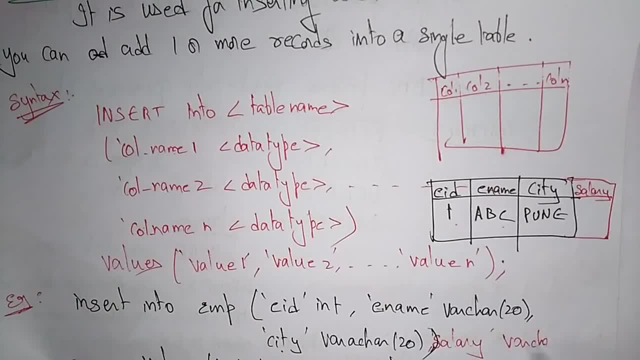 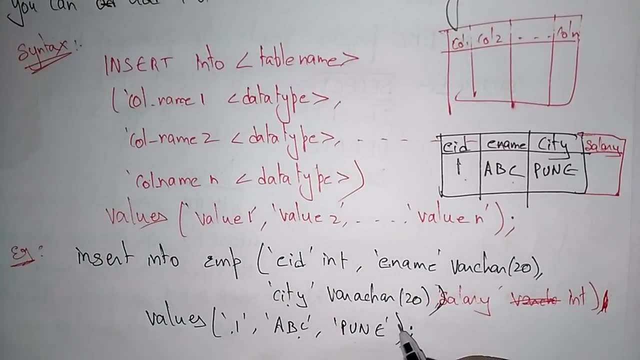 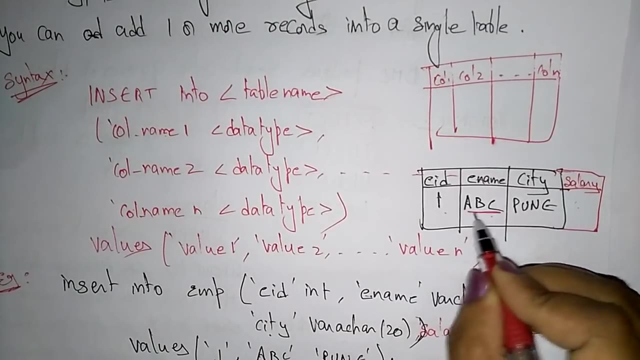 salary: varkar, so not. salary is only integer int. okay, okay, so now. so here: previously i entered some value here, or i didn't enter anything. now i want to update the person who is having the abc name. so here: update: employee set salary is equal to twenty. lasting. you have to set salary as twenty thousand where e name is abc, so here abc is equal to abc 25ád. you have to set salary as twenty thousand where e name is abc, so here abc is like in the table factory, let's fresh name of a facility. so this is a party functioning kind of, or if i want to. 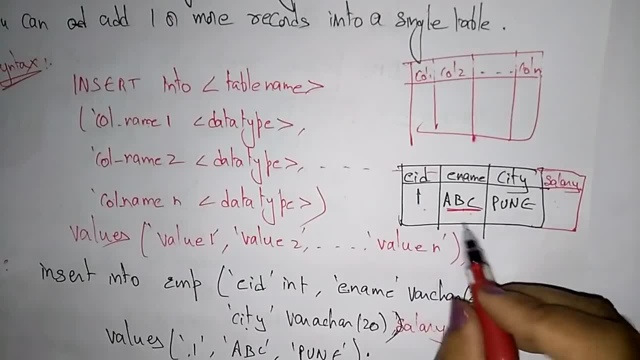 the actors and pay for theuros to be able to get free on the reserve. the work will be paid. oversize or a table cost in place of 므 here, stratégically, should not be included. so here secretary for setting the new travel schedules shall not. Air breeze will be obtained before to resume any issues. 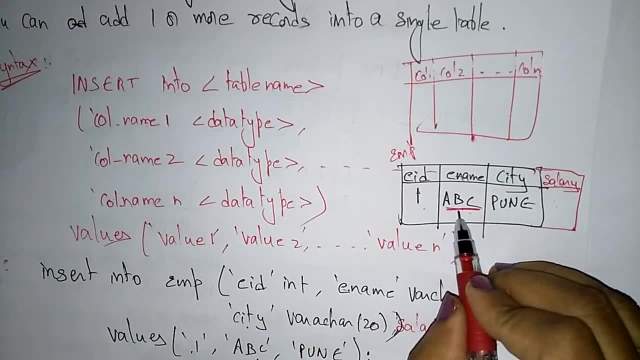 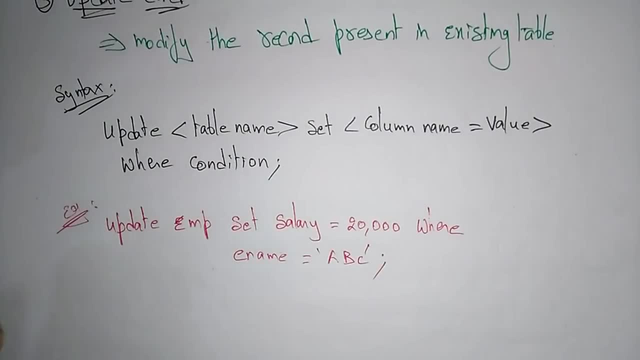 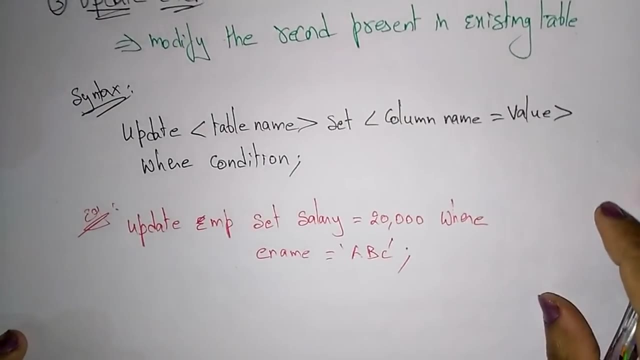 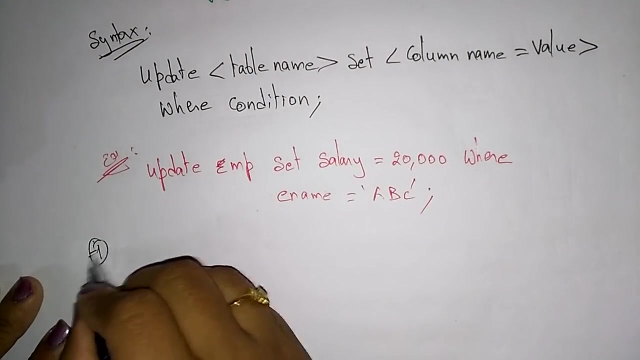 is in the employee table. abc is the e-name. i want to set salary 20 000 to this abc person. so this is how you have to use the update command. now coming to the last command in the data manipulation language. so that is the delete command. so the fourth one is: let me take another. 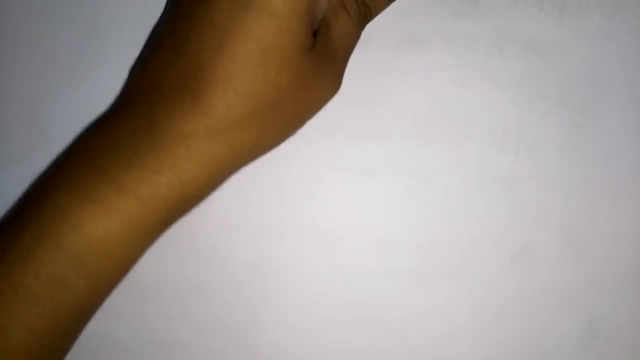 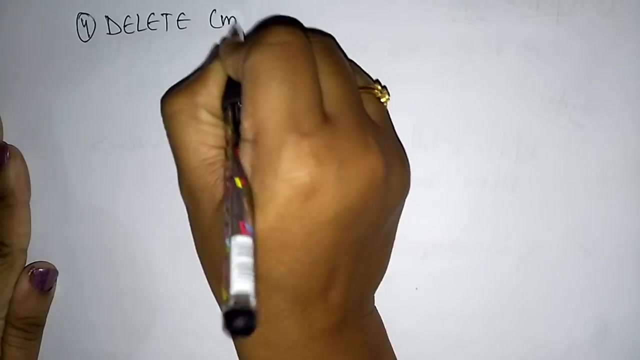 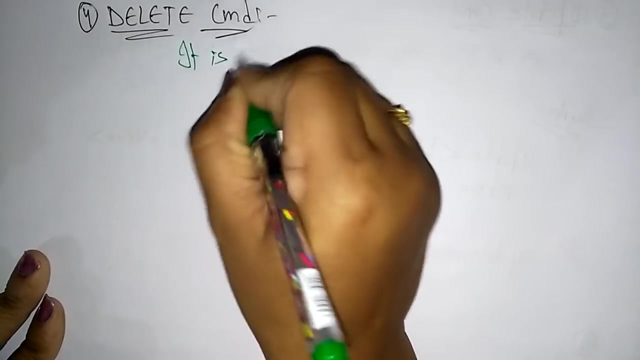 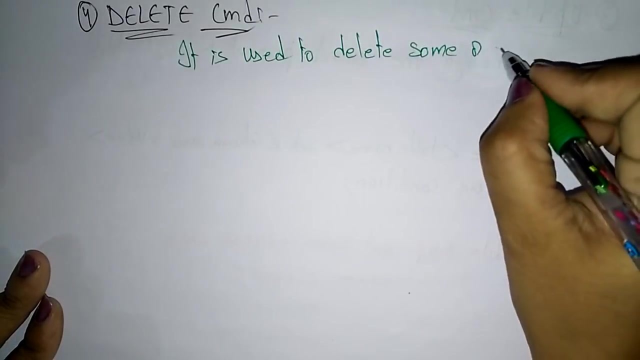 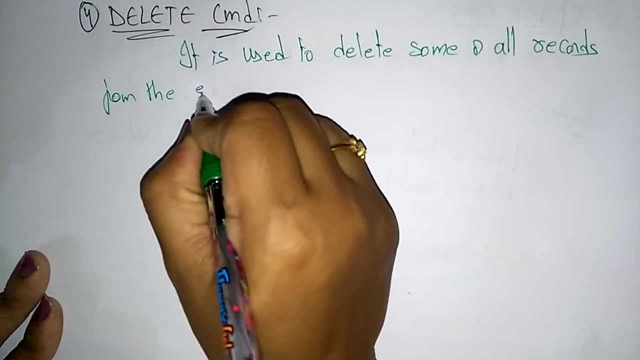 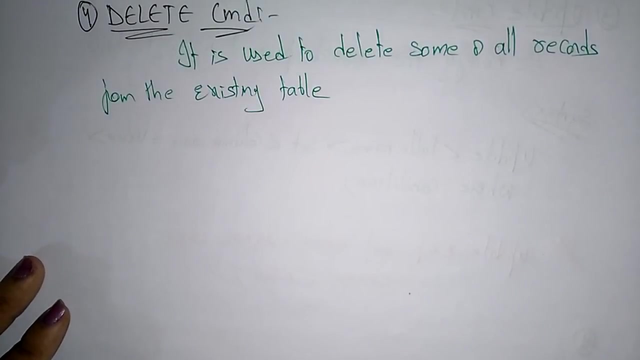 people. so the fourth command in data manipulation is delete- delete command. so what is the use of delete command? it is used to delete some or all records from the existing table. so the delete command is used to delete only the records that are present in the table. so it delete all the records or only some if the condition, if based on the condition it deletes. 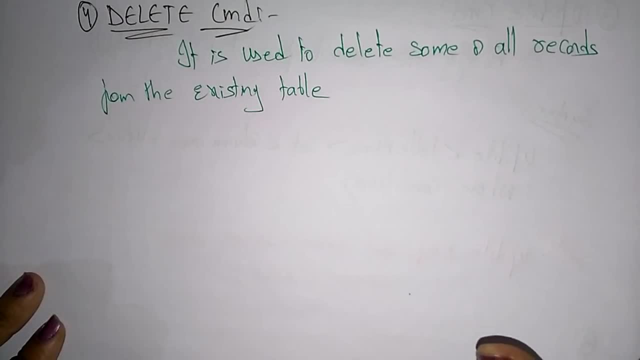 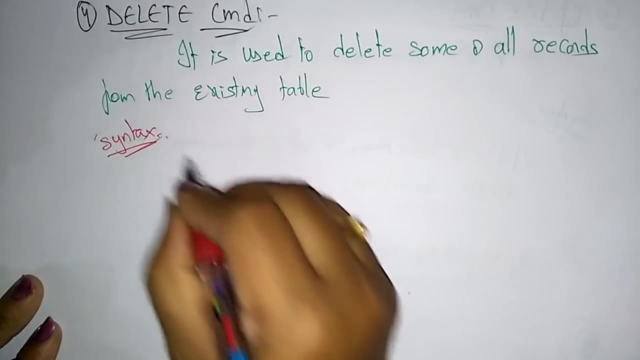 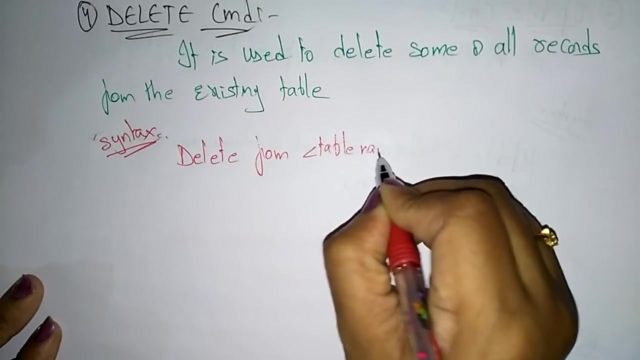 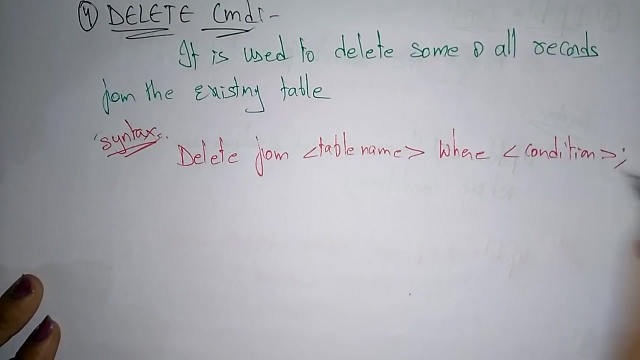 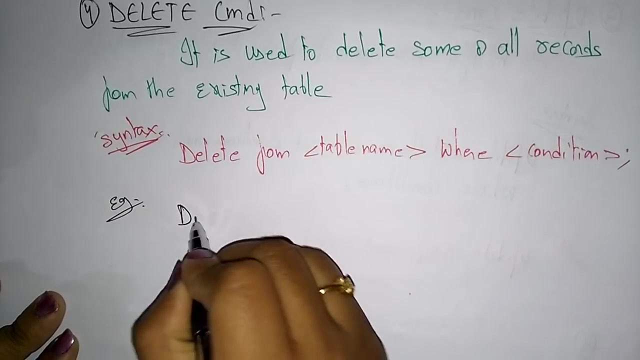 only the some records or and it deletes entire records in the table. so the syntax for this is delete from table. i have now deleted a given the label name and are using it nowwhat I mean is the int. now, what we've done is to delete content based on employee table name, say condition. 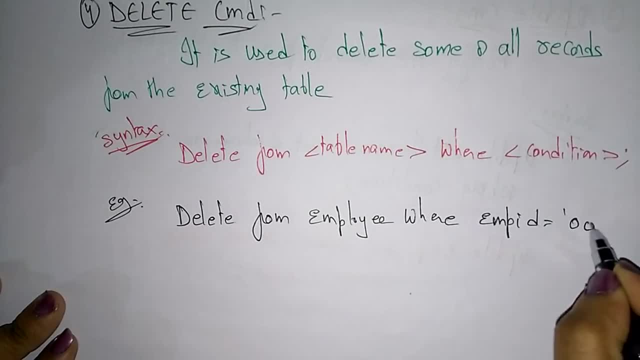 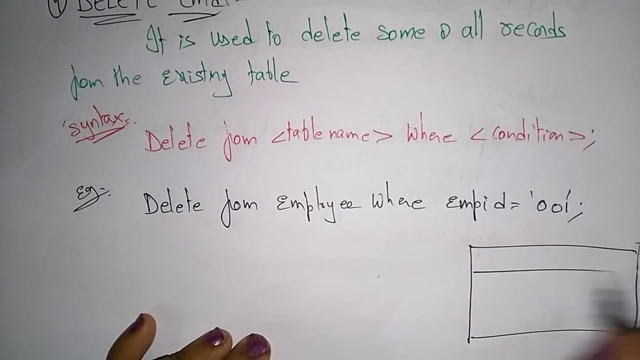 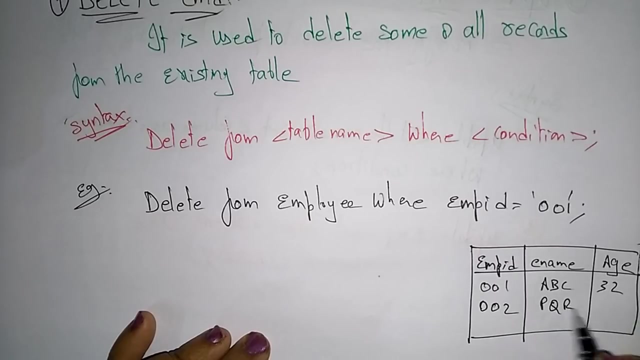 this is a syntax, now letus, see the example for this. delete from employee table. So suppose the table consisting of employee ID, employee name, age, Suppose 001, ABC, 32.. 002, PQR 35.. 003, XYZ 36.. 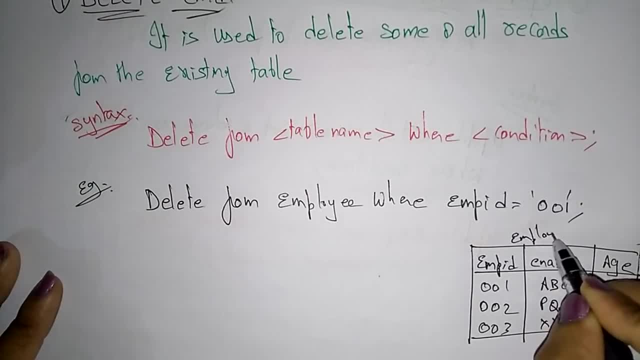 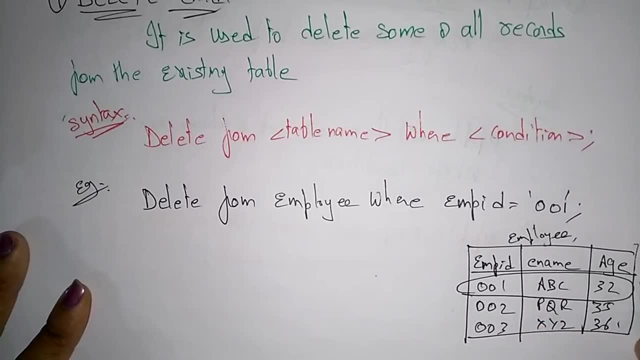 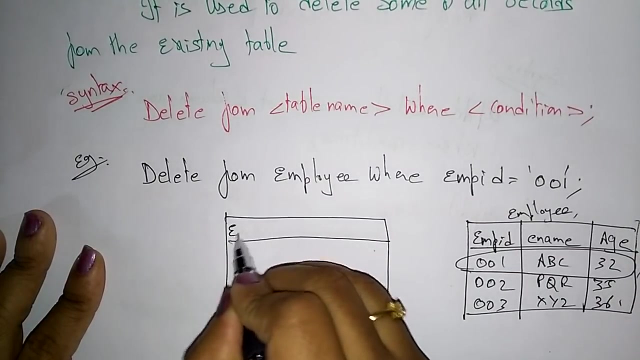 So this is a table of employee. So now when I use this command, delete from employee where employee ID is equal to 01.. It delete this complete row. Now the table. the new table will be consisting of only two rows. 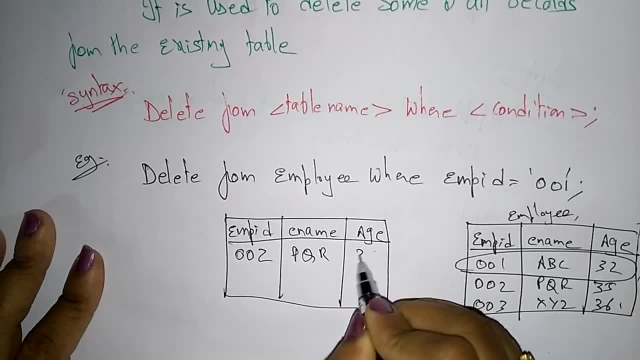 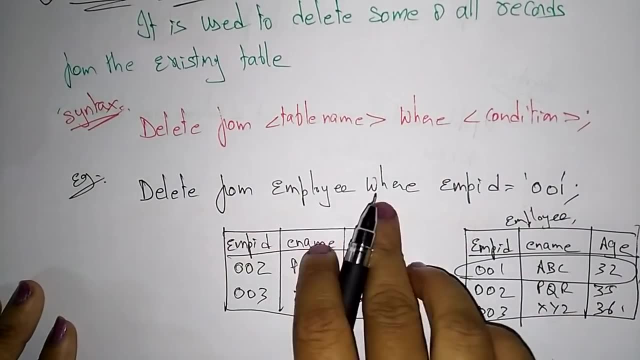 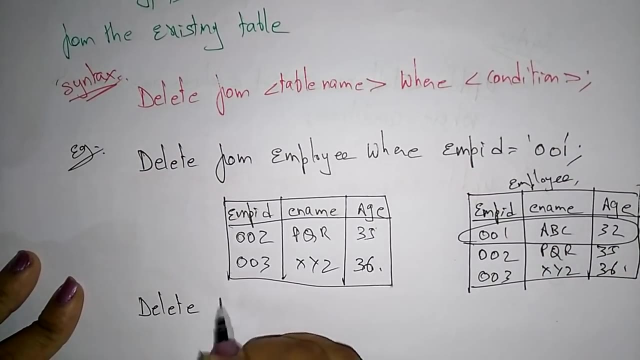 002, PQR 35.. 003, XYZ 36.. So delete from employee where employee ID is equal to 001.. Suppose, if you write just delete from employee Without mentioning the condition Means, if it does not write the where condition, then all rows will be get deleted. 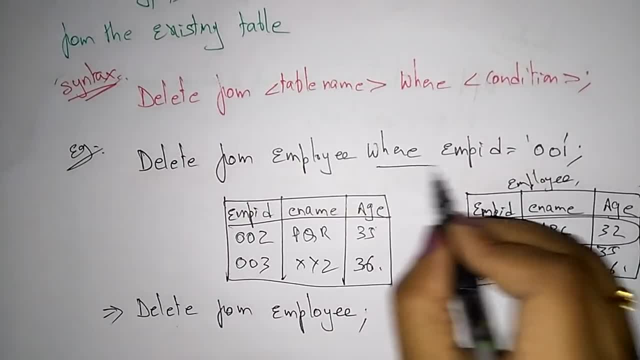 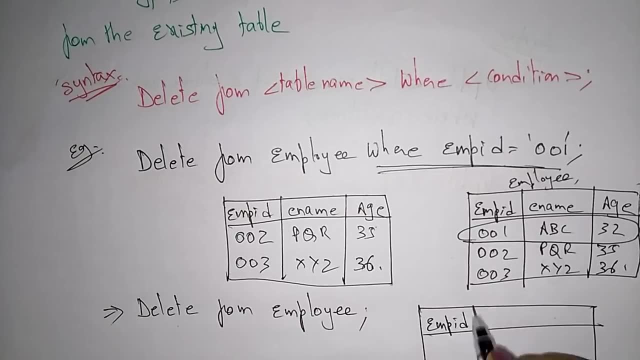 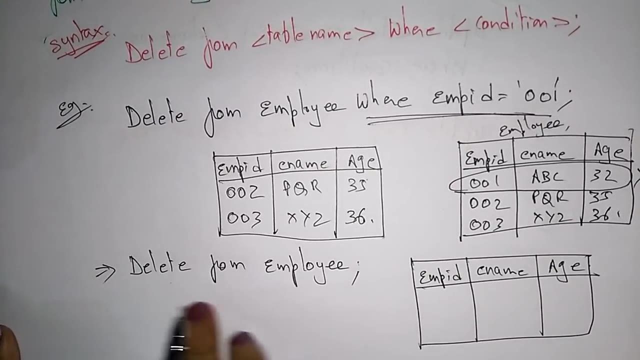 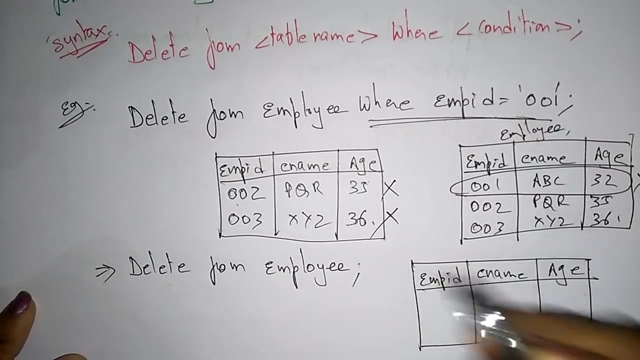 So if you write only delete from employee If you did not mention the condition, it deletes all the rows in the Employee table. now the table becomes like this: without values because I delete. I write the SQL query as delete from employee means it deletes all the rows that are present in the employee table. 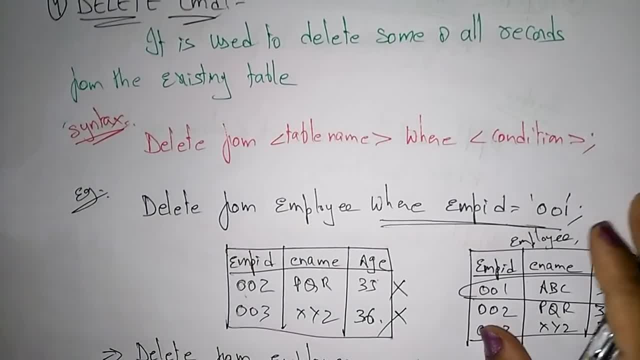 So this is about the different data manipulation language commands. Thank you.